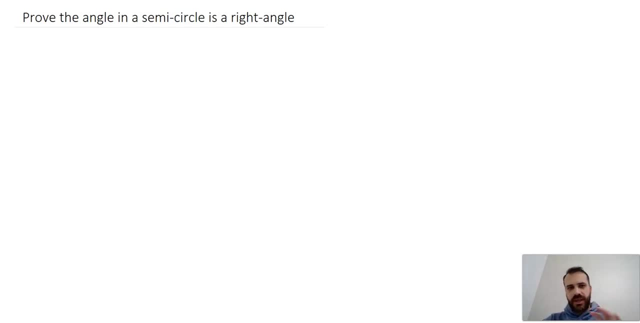 So we're getting into geometric proofs here, and this is some of the most ancient and realist maths out there. Now let's cast our mind way back to like ancient Greek times. Think about this kind of action: A bunch of guys standing around in robes with sticks, drawing geometric figures in 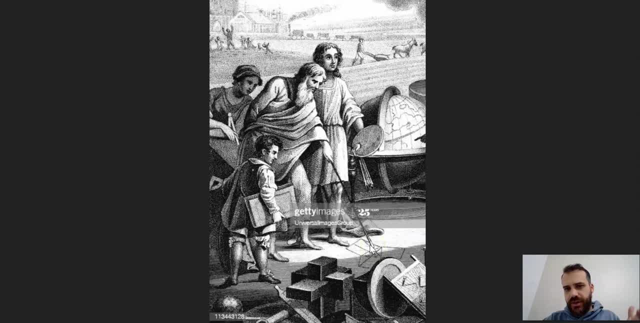 the sand and trying to come up with mathematical ideas. Now, the Greeks didn't have a monopoly on this. Babylonians, the Chinese, the Arab world, like all over the world, they were doing things like this. People are curious. they want to know this stuff, So here's one thing that they might. 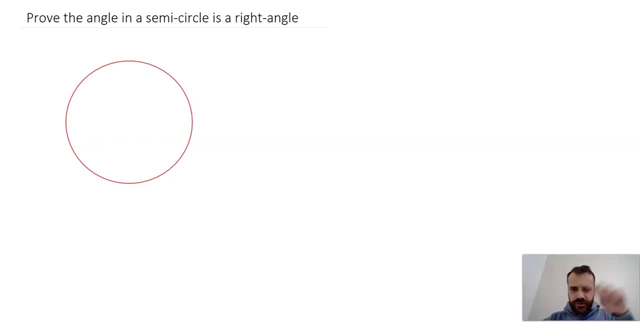 have scratched into the sand. So our hero draws a circle in the sand and then he cuts that circle in half. Then the next thing he does is pick a random point somewhere else on the circle and now he takes that random point and he draws lines from here and from here to that random point and 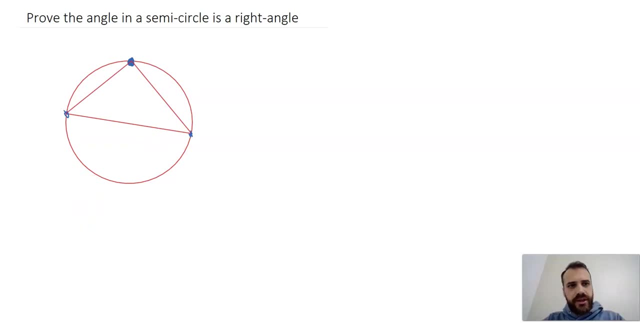 then he shows this drawing to all of his friends and he thinks, hey guys, don't you think this looks like a right angle? And everyone's like, yeah, that kind of does look like a right angle. And he says I wonder if it is. And then he makes something called a conjecture: This is a 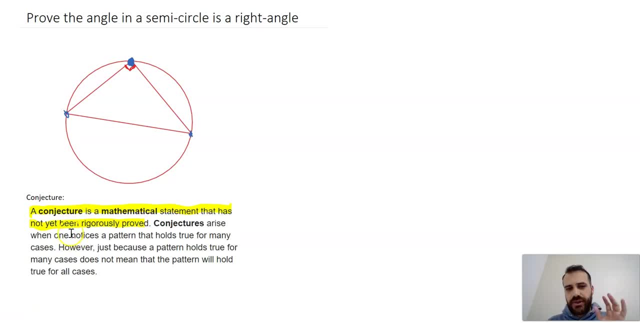 pretty decent definition of a conjecture. It's a mathematical statement that has not yet been rigorously proved. He says: right, I've drawn this semicircle here, I'll just put a center in there, so you know that this is a semicircle. I've picked a random point and it could have been any point. 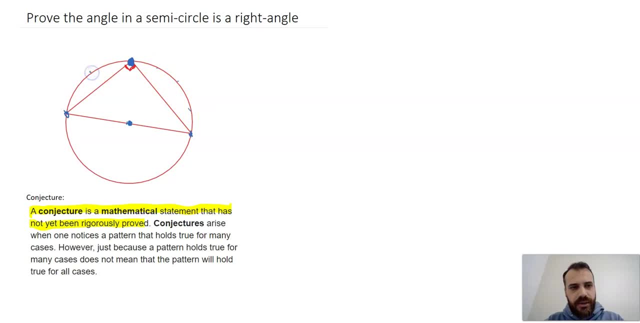 I could have picked this one, I could have picked that one, I could have picked that one. I could draw two lines to that point. I'll always get a right angle, And at the moment it's just a conjecture. and then he sits down and proves it, And that's what we're going to do here. We're going. 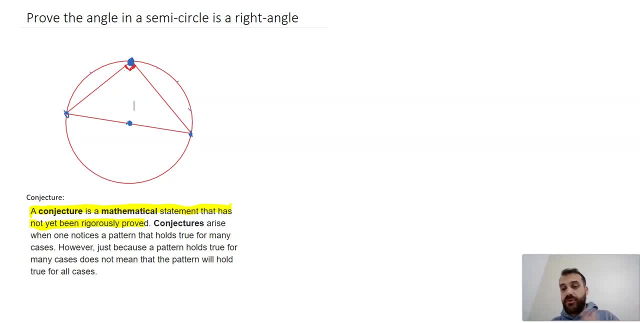 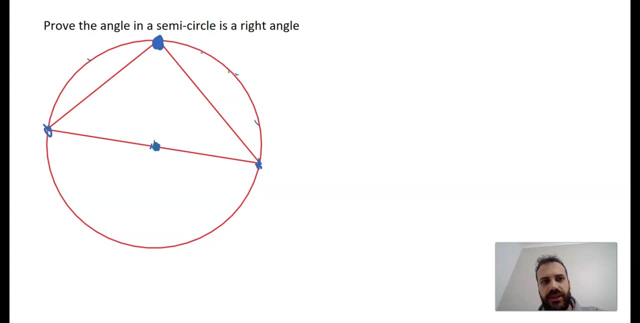 to prove it Now. you might want to pause the video here and try proving it yourself. All right, so when I'm proving this, it's going to be important to be able to refer to sides and angles and things like that. So I'm just going to label this up a little bit. I'll call this point A. I'll call this. 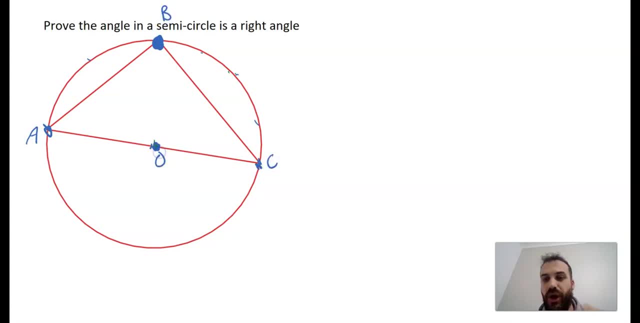 point B. I'll call this point C, I'll call this point D. I'll call this point C, I'll call this point D, I'll call this point C And I'll call this point O. O for origin, And I'm going to do something. 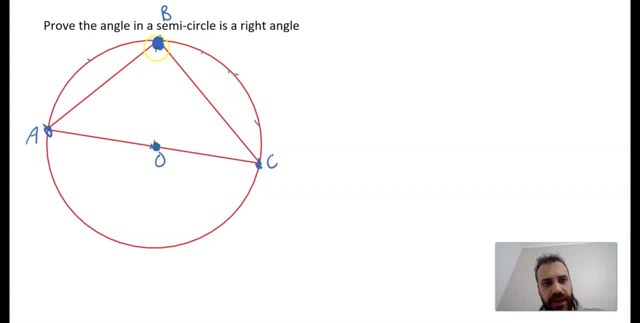 called a construction. So I'm going to draw a line from B to O- And constructions in proofs are really, really useful- And I'm going to write that as I'm doing it. All right, so I've constructed a line B O. Now this is a circle and this is the center. So what can we sort of? 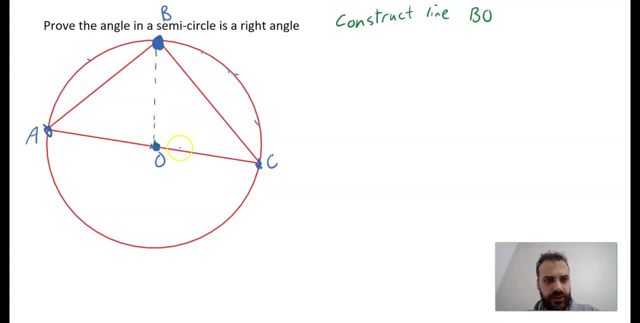 ascertain about this bit here Or this bit here Or this bit here. They're all different. So I'm going to call this point C And I'll call this point O? O for origin, And I'm going to write that as I'm doing it. All right, so now that I know that A, O, B, O and C? O are all, 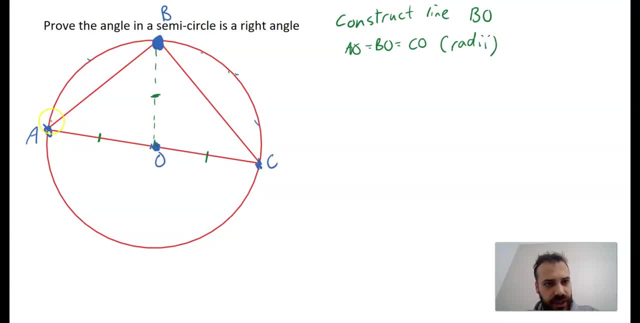 radius. So I'm going to call this point C And I'm going to write that as I'm doing it. All right, I can look at this triangle here, Triangle A, B, O, And I just write a triangle in there And look. 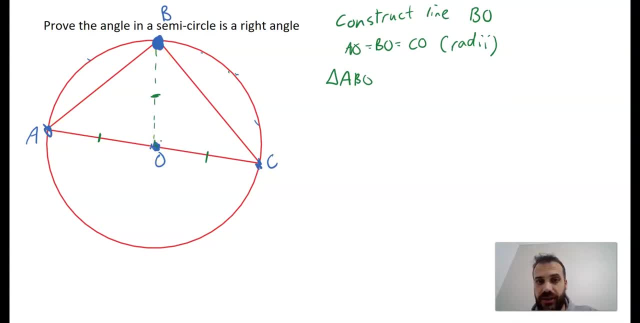 at triangle A- B O. It's an isosceles triangle And triangle B or C O B or B O C. however, you want to say, it is also an isosceles triangle. So triangle A, B O and triangle B O C are isosceles. 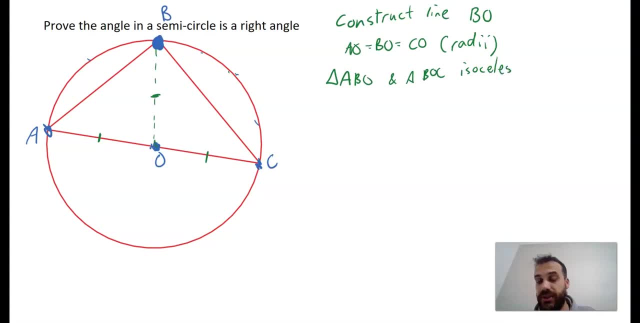 And the way that we know that they're isosceles is: the two sides are the same. Okay, now, what can we do from here? Well, let's call this angle X Right now. if this is angle X B A O, So we can say that angle B A O is equal to angle A B O, This angle here. 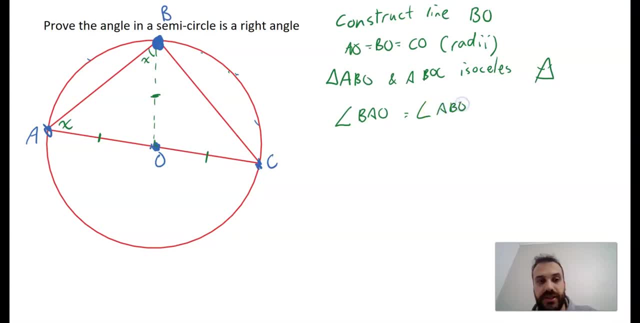 So angle A, B, O, And the reason they're equal is because they're isosceles. Okay, two equal angles, Two equal, Sorry. two equal sides, Two equal angles. And we can do exactly the same thing with this triangle here. I can call this Y And I can say that angle O, C, B is equal.